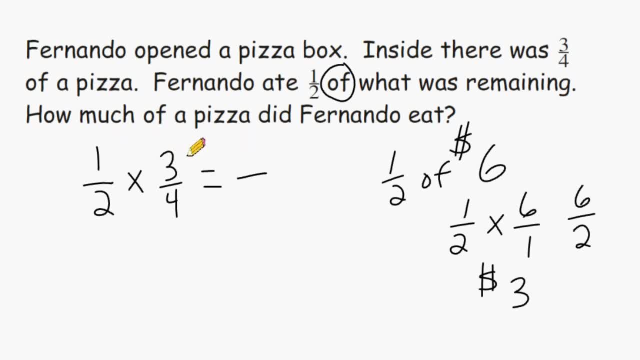 set up. all we have to do is multiply straight across. One times three is three, and two times four is equal to eight. So we would say that Fernando ate three eighths of a pizza. Now, another way that we can think about this problem is to draw a pizza and then break. 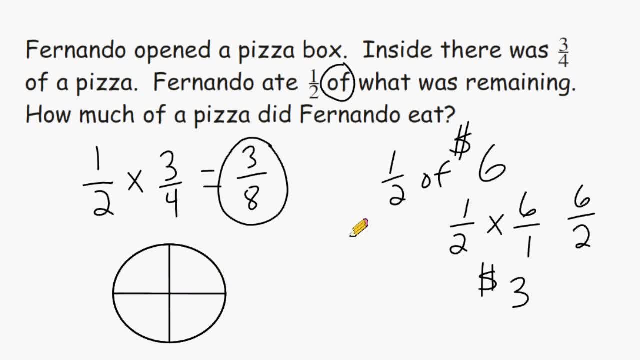 that into quarters. So when Fernando opened up the pizza, there was three fourths of the pizza remaining. So we're going to shade three fourths of that pizza and out of those three large slices, Fernando ate exactly half of those slices. Now notice that you cannot cut the number. 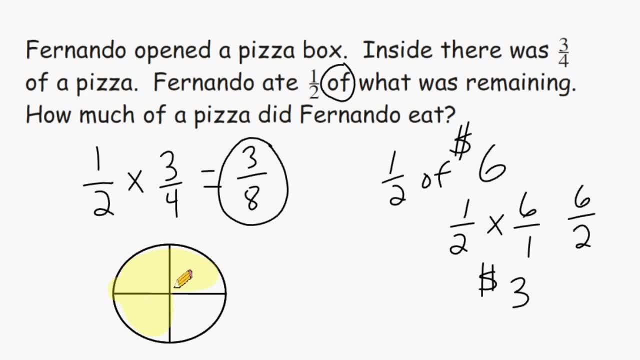 three equally in half. but what we can do is we could cut each one of these three pieces in half. So if we cut each one of these pieces in half, what we are doing is forming eighths, And we're going to take this part that's already eaten and just cut that in half as well. so 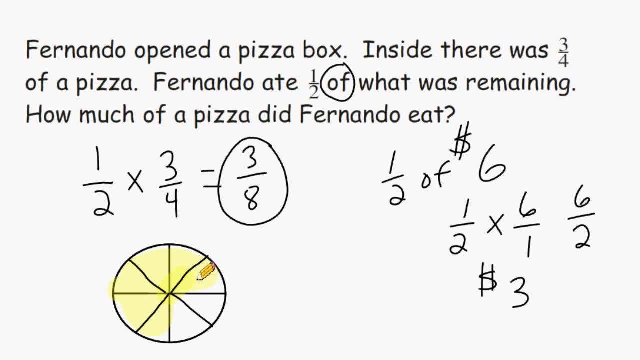 we can see that we have eight equal parts. Now that we know that there are six eighths remaining, we can take half of that, because Fernando eats half of six eighths, which would give us one, two and three eighths. 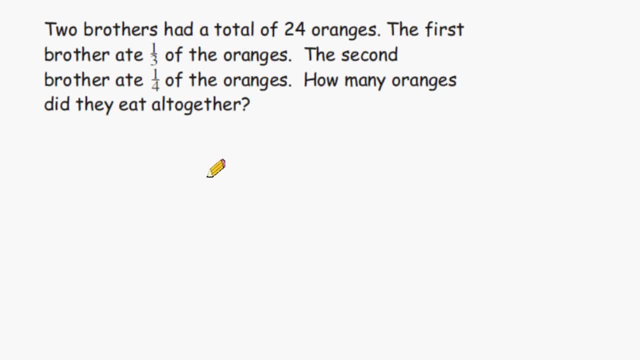 This problem reads that two brothers had a total of twenty-four oranges. The first brother ate one third of the oranges. The second brother ate one fourth of the oranges. How many oranges did they eat all together? Well, one strategy to approach with this problem is to figure out what one third of twenty-four 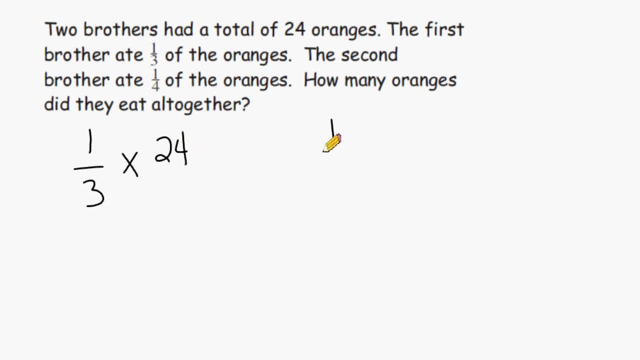 oranges is equal to. And also we have to figure out what one fourth of twenty-four oranges is equal to, because the first brother ate one third of all of the oranges and the second brother ate one fourth of all the oranges. And once we figure out how many oranges each, 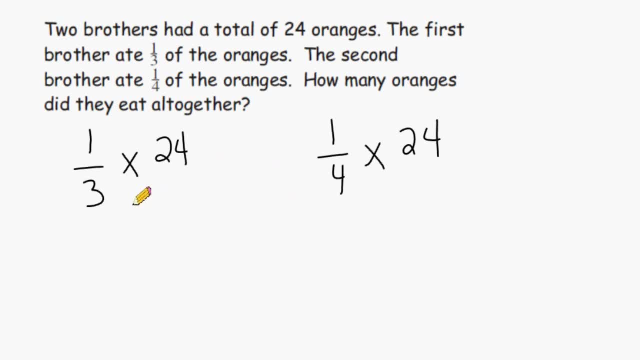 brother ate. we can add those quantities together. Well, one third is the same thing as dividing something into three equal parts. How many oranges did the first brother eat? Why is the fourth brother eating one third of the oranges and the second brother eating one? 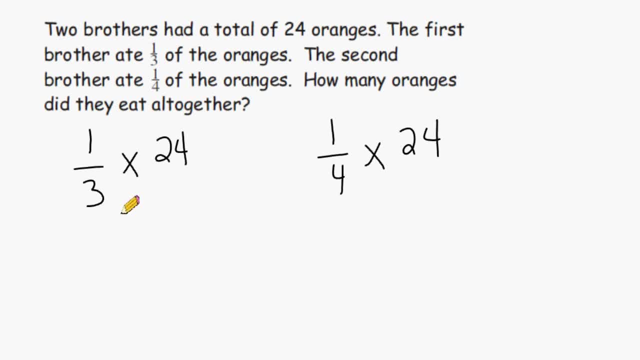 hearts. So essentially this problem can be mental math. So let's just take 24 and divide that by 3. That would give us a total of 8 oranges. And to figure out what 1 quarter of 24 oranges is, we could take 24 and divide that by 4, which would give us 6.. So the first 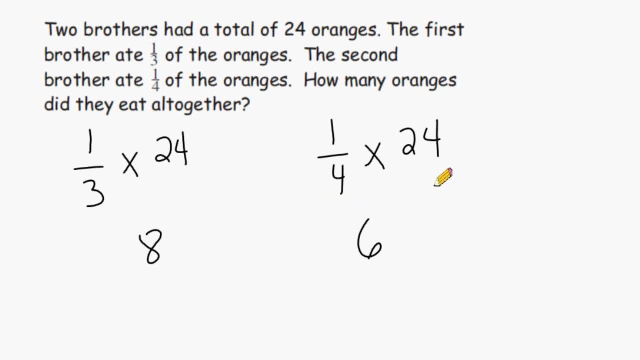 brother ate 8 oranges and the other one ate 6 oranges, for a total of 14 oranges. Now if we were to carry out our multiplication, or do 1 third times 24, we will see that that also gives us a quantity of 8.. So if we multiply the numerators together, we would come up with: 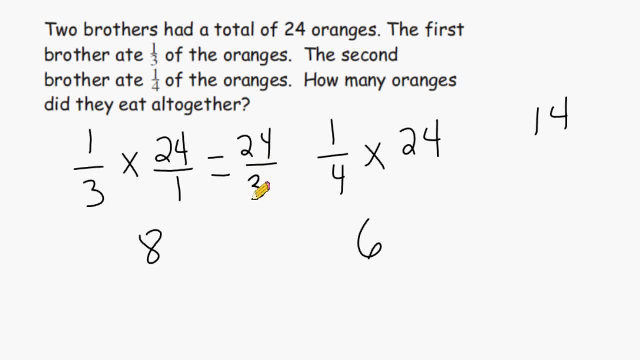 24.. The denominators would yield a product of 3, and that gives us an improper fraction that we may simplify by doing 24 divided by 3, which is 8.. And for 1, fourth of 24,, we can multiply the numerators, which gives us a product of 24.. 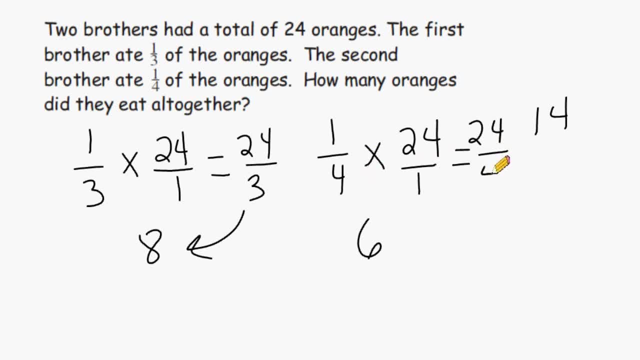 And on the bottom we have 4 times 1, which gives us a product of 4.. And 24 divided by 4 is equal to 6.. So we can add 8 and 6 together and that would give us a total of 14 oranges.